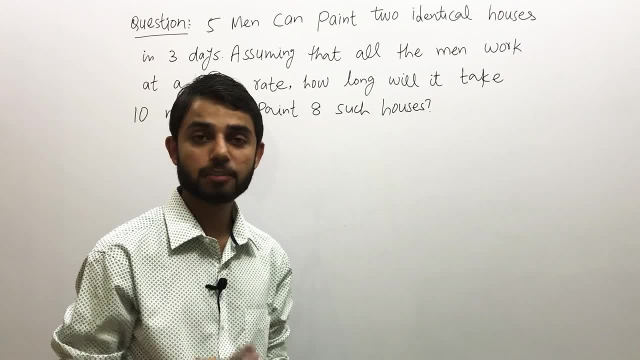 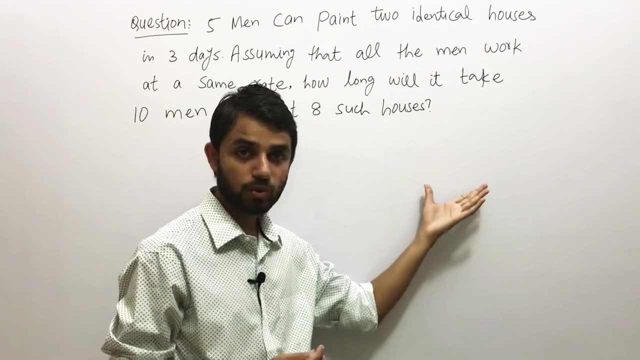 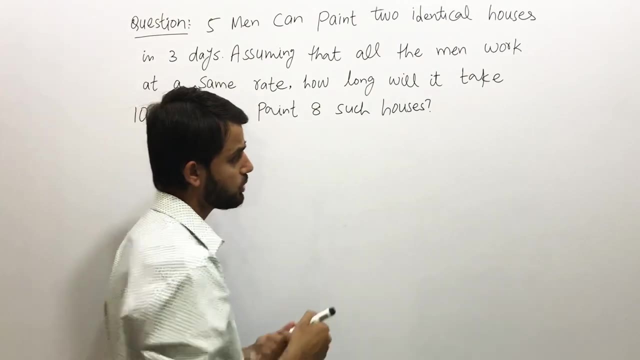 Number of houses is your second variable, and the third variable is number of days. So we are having the 3 variables. So let me tell you in general how to cope up with these kind of a problem, and then we will apply that method to this particular question. Let's suppose that we are having the 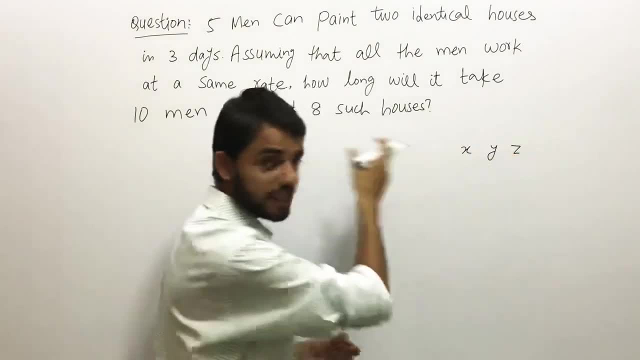 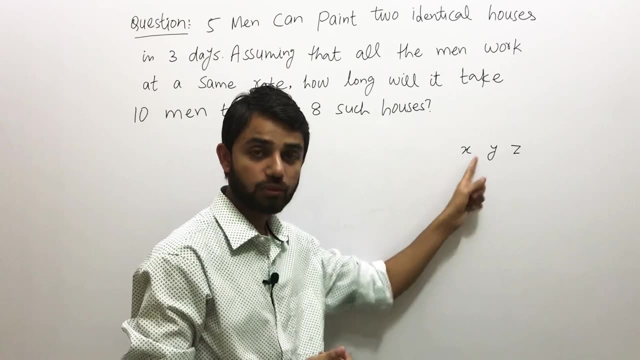 3 variables- x, y and z- in these type of questions, and then we will try to keep one as fixed and then we will solve the other one. So let's say that we are having the 3 variables x, y and z in these. 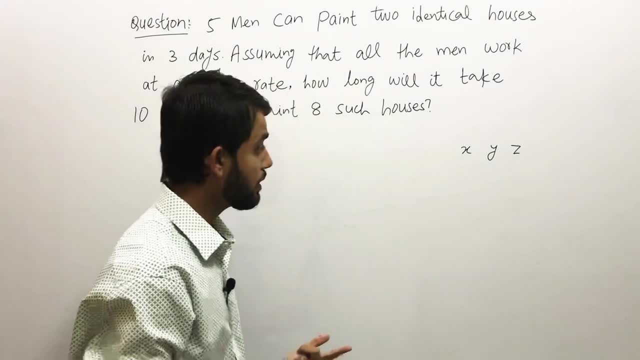 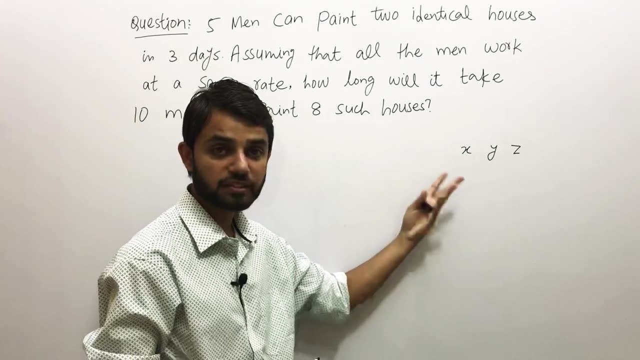 type of questions, and then we will try to keep one as fixed, and then we will try to keep one as fixed and we will try to find out the relation between them. So the question is that how we will get to know that for which variable you have to keep it as a fixed quantity. Now read this question again. 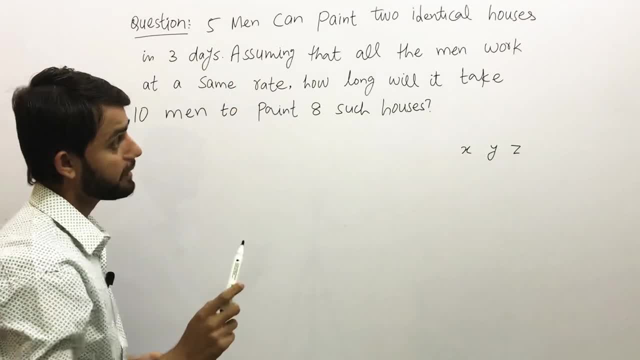 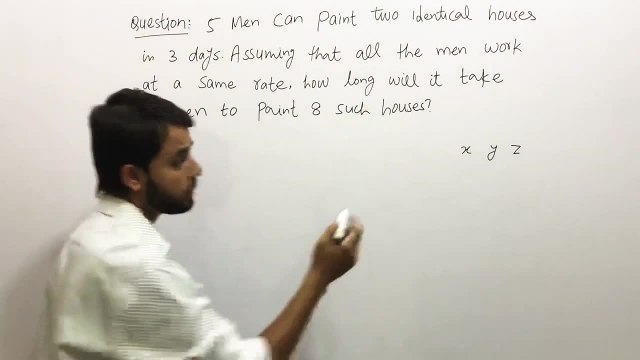 and find out which one. 5 men can paint 2 identical houses. Let's say that men is your x. identical houses, number of houses is your y. Alright, let's represent with men. and then we are having the 3 variables x, y and z in these type of questions. So let's say that we are having 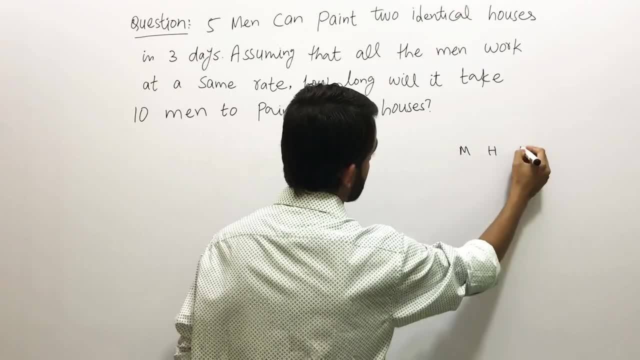 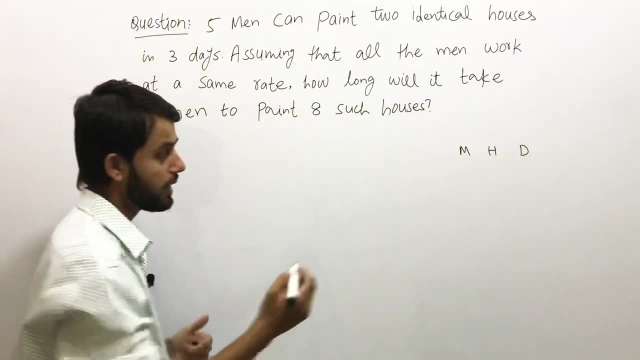 number of houses and then we are having the number of days. So m, h and d Men are given to you, 5 men over here and the 10 men over here. So men are basically we are having 2 times Okay the houses. 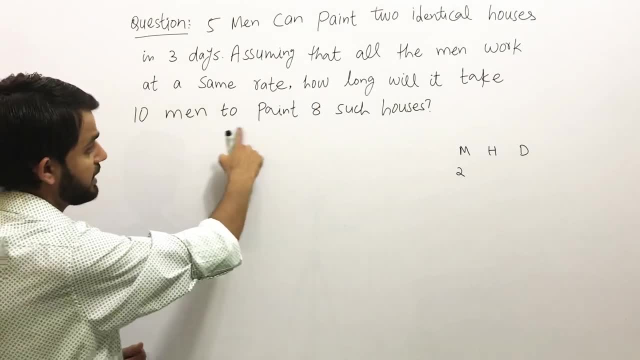 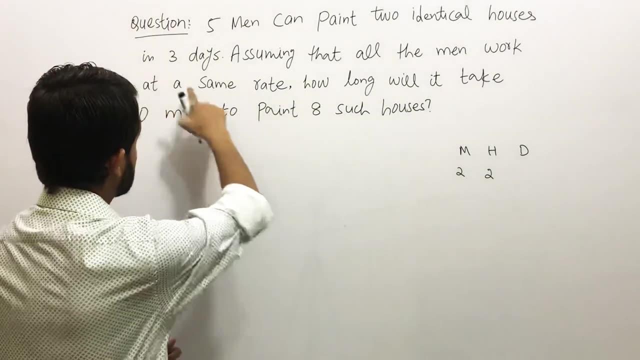 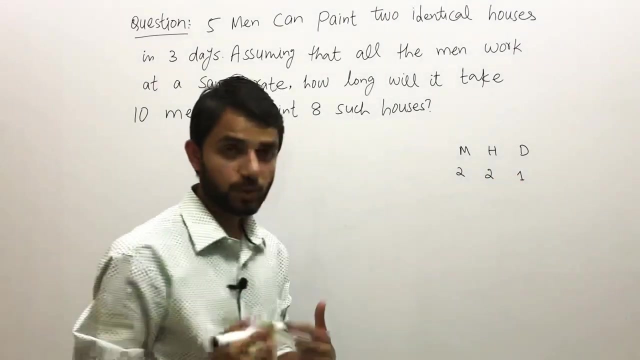 initially we had 2 identical houses and then 8 houses, So they are also 2 times. have been given to you in the question Now 3 days, and then how long will it take? The number of days are being given to you 1 time, So whatever value have been given to you 1 time. obviously that's what you need. 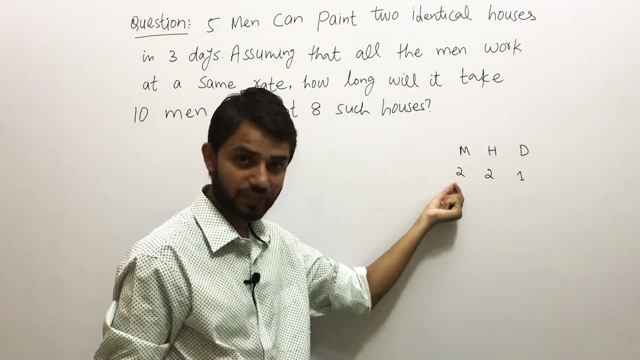 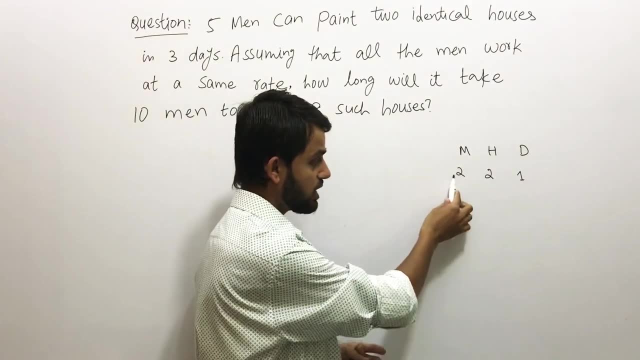 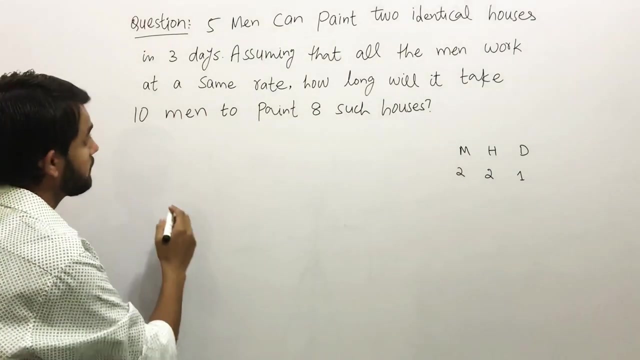 to find it out From these 2. you will keep 1 as a fixed quantity and then you will try to solve it. for the next 2, and then the one you kept initially as a fixed quantity, you will involve this with the other one and then you will solve it out. Okay, let's begin with the solution. So we are having 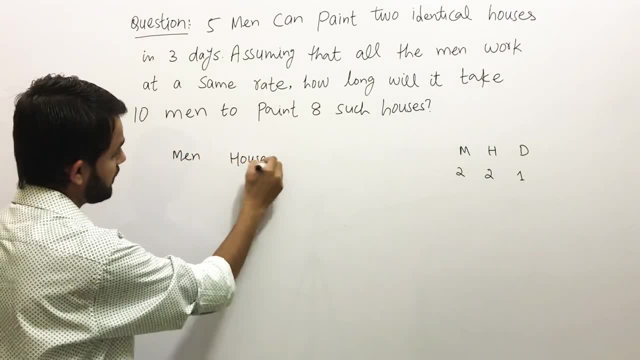 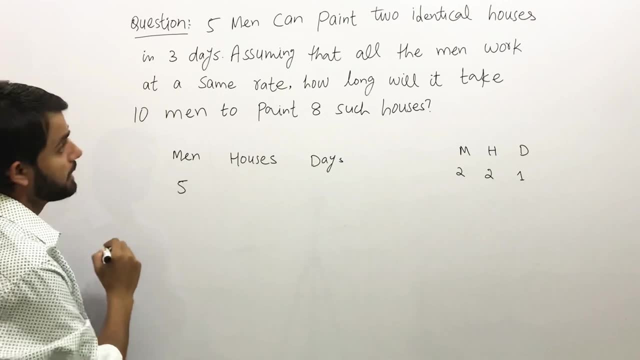 men. we are having number of houses and we are having 2 men over here, So let's say that we are having number of days. Now the question says: 5 men can paint 2 identical houses in 3 days. So what? 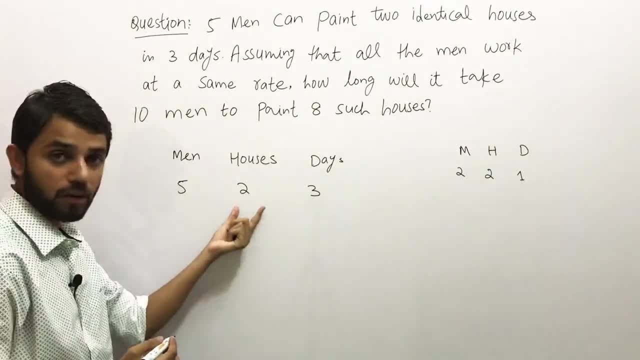 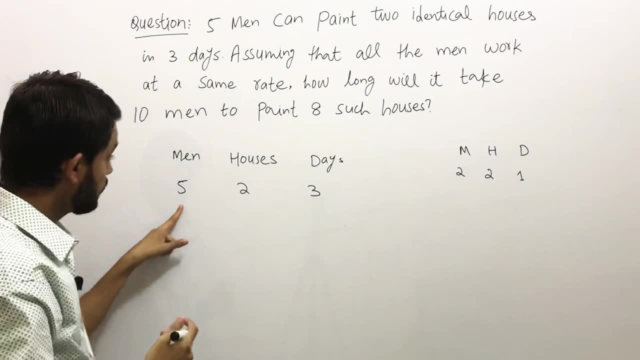 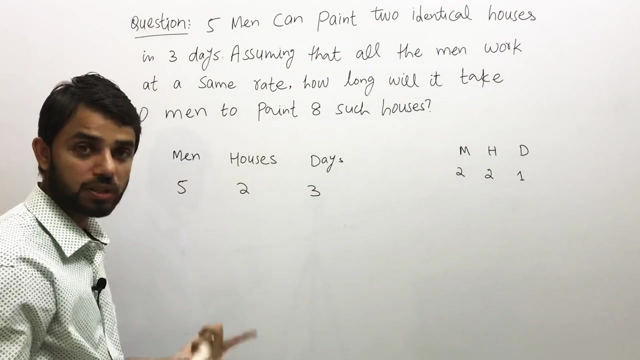 I am going to do now. I am going to keep number of houses as a constant quantity and then I will try to find out the relation between men and days. Okay, so now you will see that if we are going to decrease the number of men, obviously number of days are going to be increased. 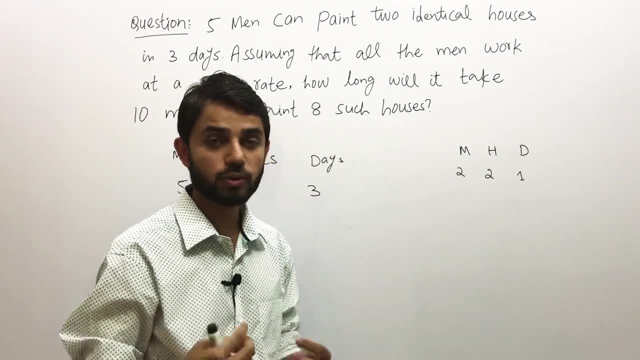 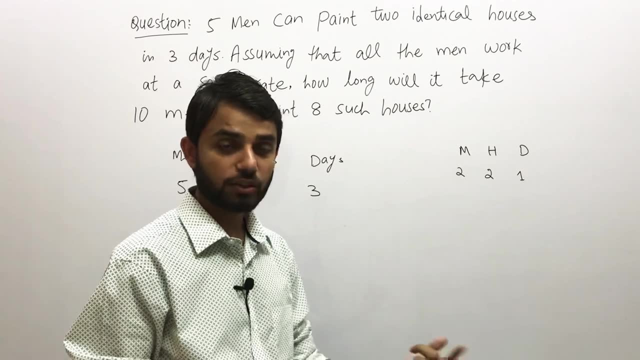 Let's suppose that me, along with my crew, who were doing a job, and that task actually requires 6 men in order to complete their task in 12 days. So if I have to do all that work all alone, so number of days are going to be. 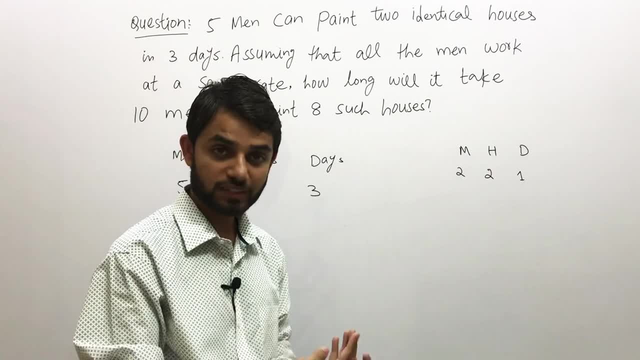 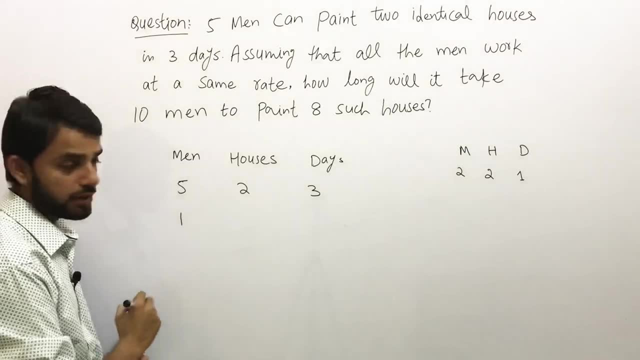 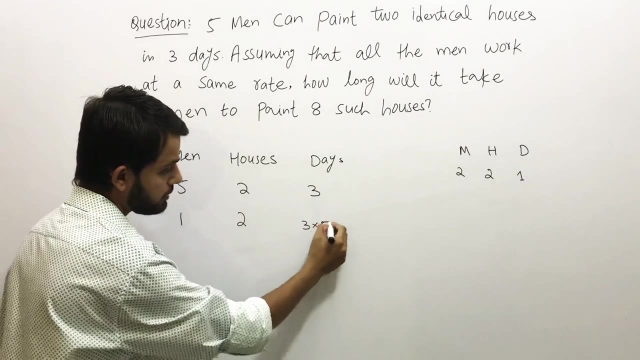 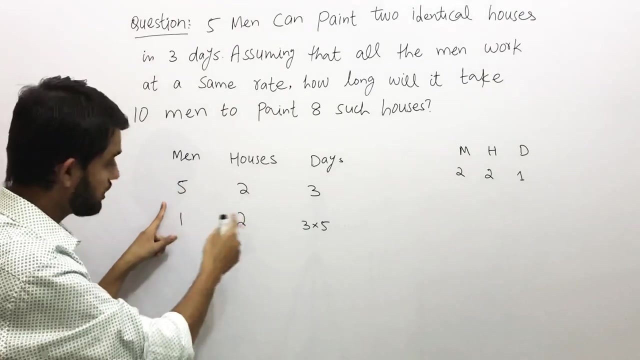 increased. So the relation between me and number of days is basically the direct proportion. The same thing over here now we will do for 1 man in order to complete 2 houses. the number of days are going to be increased 3 times 5.. Okay, so because men and days are in inverse proportion, if we decrease the number of men, 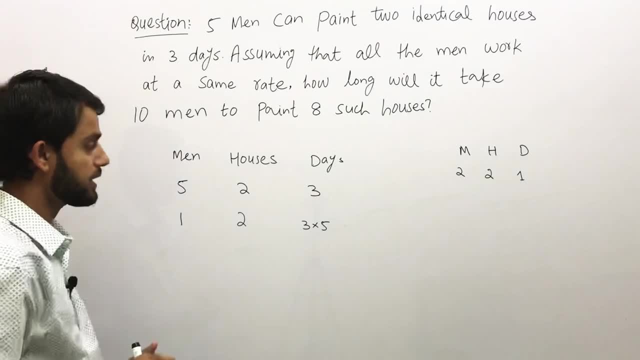 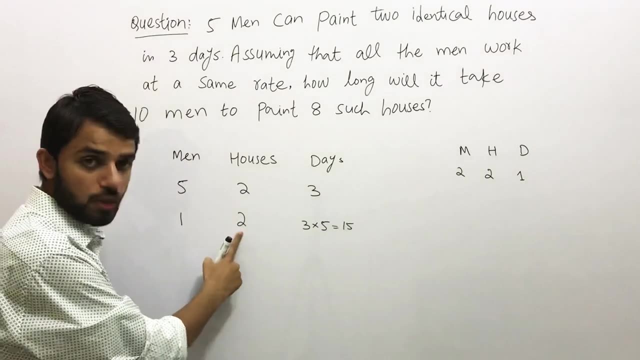 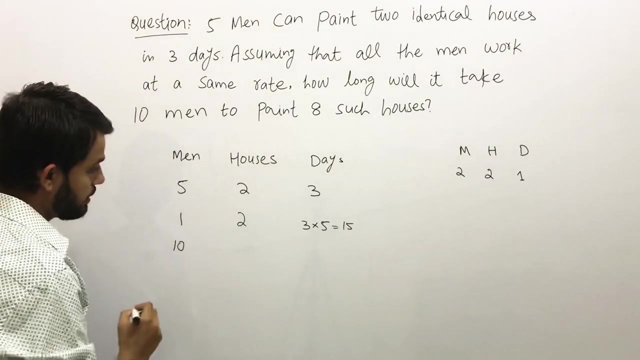 number of days are going to be increased, So that is why we are multiplying with that: Okay, so, which is actually 15.. So, for 1 man, in order to complete 2 houses, it will take 15 days. Now we will find out that for 10 men, in order to 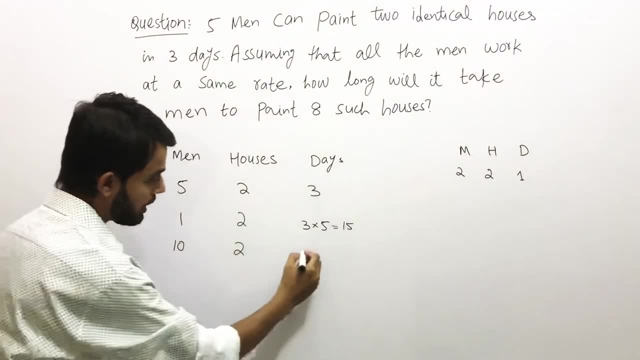 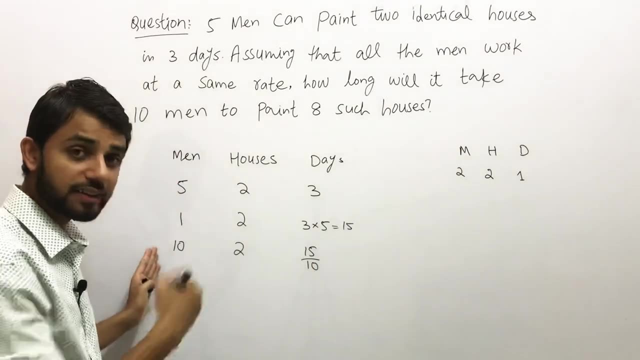 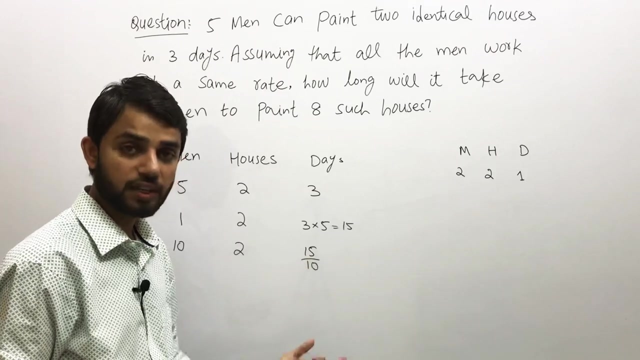 complete 2 houses. how much days it will require? 15 divided by 10.. Now why I am dividing with 10? Since the number of men are increasing, the number of days are going to be decreased. The only possible way you are going to get the decreased days if you divide with the number. So that is why we are 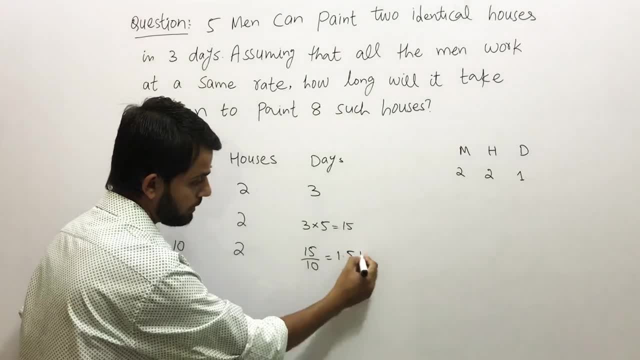 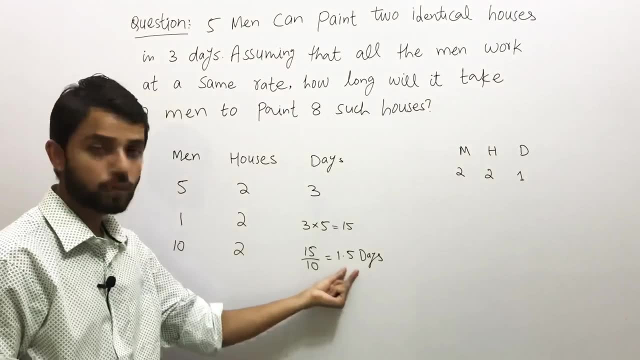 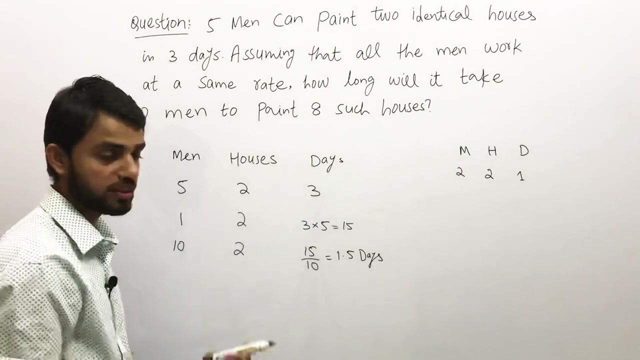 dividing with 10. So we got 1.5 days. So it means that for 10 men to paint those 2 houses it will take 15.5 days. So in this case, in the first case, the relation between men and days was inversely. 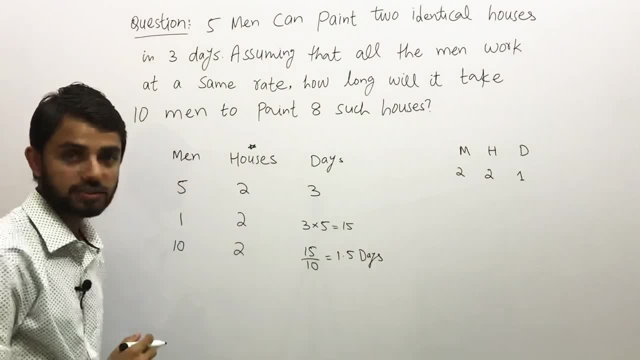 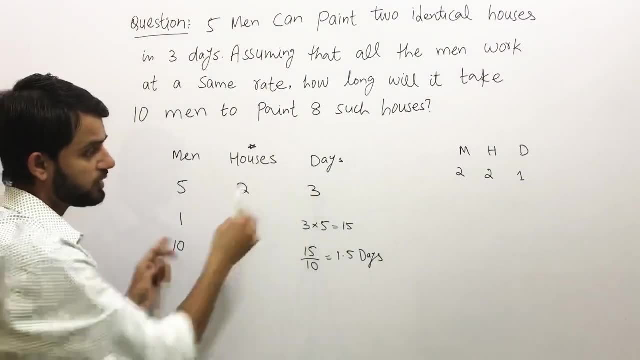 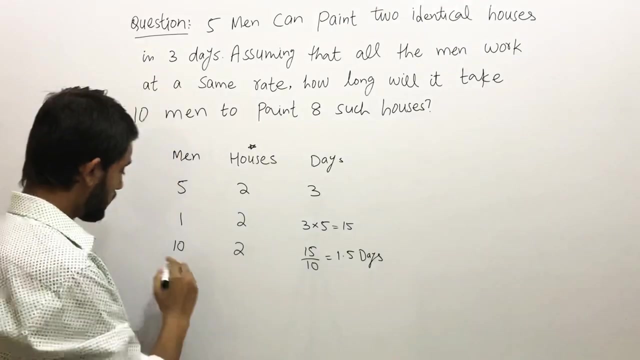 proportional and we will keep this quantity as a fixed or as a constant. Now, we will keep men as a constant and then we will find out the relation between houses and number of days. Whatever answer you got from this part, you are going to start it from here. So, men?